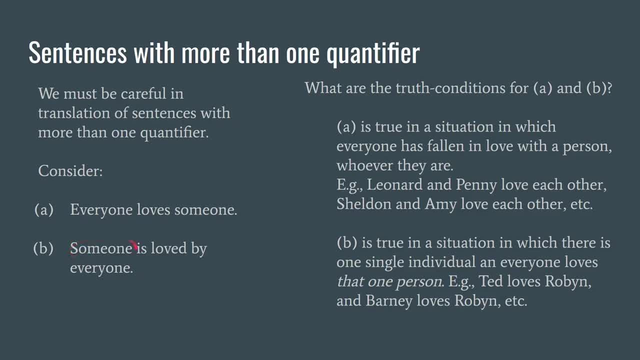 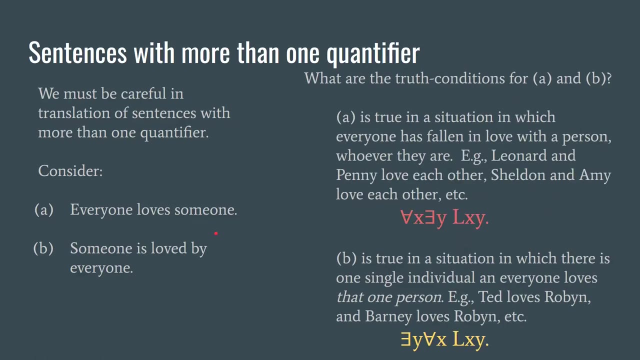 different, Whereas what B is communicating is that there's some one person and everyone loves that one person. A and B represent two very different situations in the world, So our logical translation needs to represent these differently. The way to do this is to switch. 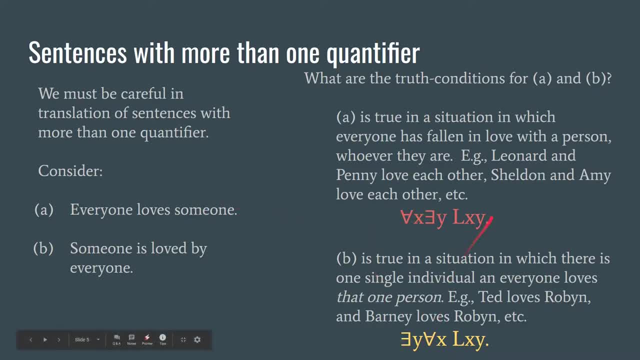 the order of the quantifiers. Notice, in both translations we have LXY as our relational predicate, but the order of the quantifiers is switched Here. at the top we have for all X, there is a Y, such that X loves Y. At the bottom, we have there is a Y, such that for 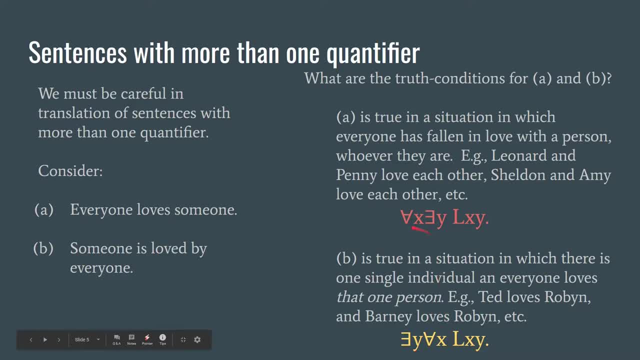 all X, X loves Y. These look very similar, but they have very different meanings. Again, for all X there is a Y, such that X loves Y tells us that everyone loves someone- Each pair might be different- Whereas B tells us that there's some one person and everyone loves that very same person. 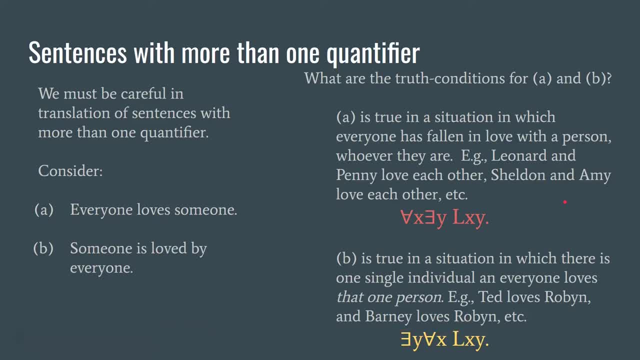 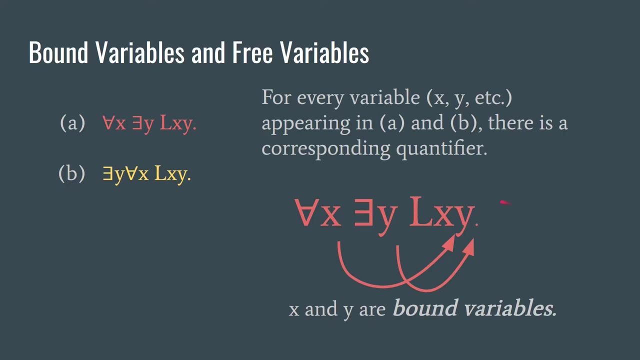 So order of so big picture here. order of quantifiers counts and we need to think about the order of the quantifiers when we're using sentences that have multiple quantification phrases in them. Now we need to introduce the notion of a bound variable and a free variable. Remember X. 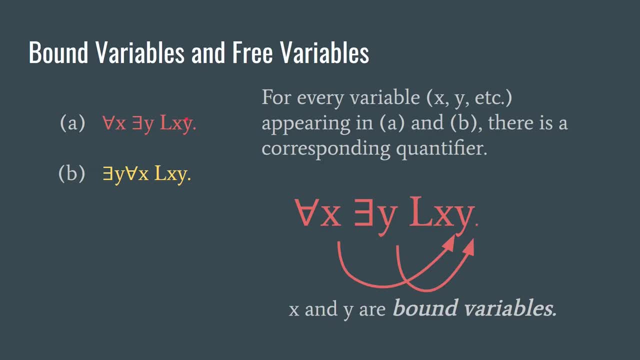 and Y are variables. They're not like A, B and C, which stand in for names of a specific person, X and Y. we don't know who X and Y are in particular. We're just saying everyone and someone. No particular object is being denoted here. Now notice that in both A and B, X and Y each have 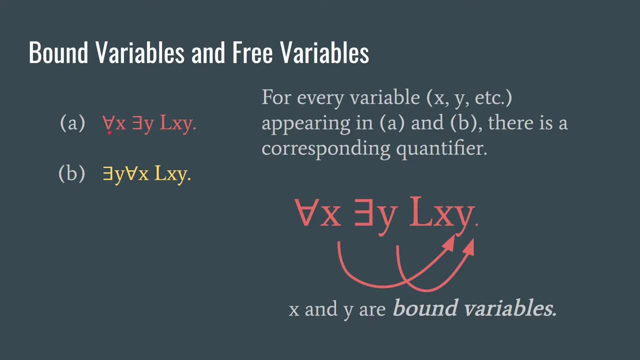 a quantifier that is binding them. That is to say, we have a quantifier attached to the and a quantifier attached to the Y. So LXY here contains no instances of free variables. All of the variables in these are bound variables. Contrast those examples with these new ones. 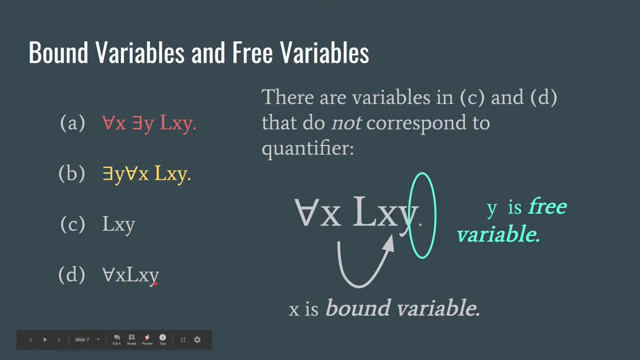 LXY and for all X LXY. Notice that in these cases, if we look at C, X and Y here have no quantifiers corresponding to them. That means that both X and Y occur free in this one. In D, however, we have a universal quantifier corresponding to the X variable. So X is bound. 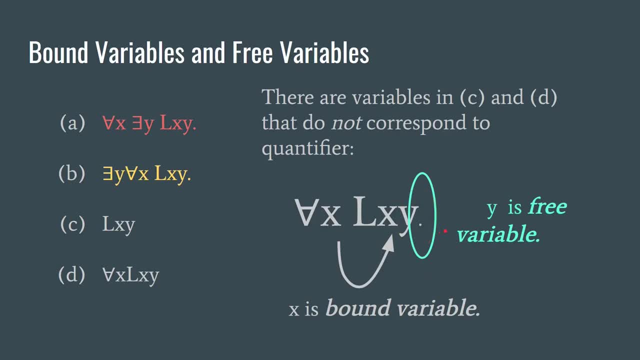 but Y is free in this case. So very important distinction between free variables and bound variables. A free variable is when there's no quantifier corresponding to that variable and a bound variable is when there is a quantifier corresponding to that variable. Unlike propositional logic, 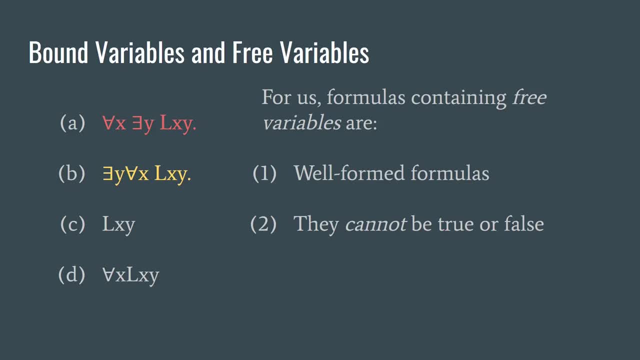 where a formula and a sentence go together. here there's a difference in predicate logic between a formula and a sentence. So C and D here both have free variables and they are well-formed, That is to say, syntactically these are perfectly legitimate. 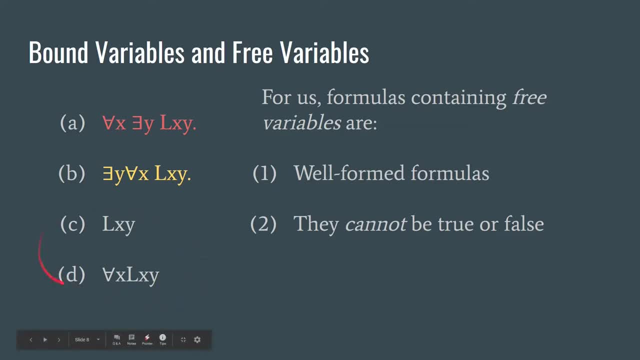 But they do not create complete sentences. That is to say, this is what's called a propositional function, not a proposition. What that means we'll say more about in the next slide. But the basic idea here is that C and D cannot be true or false. We don't know how to evaluate. 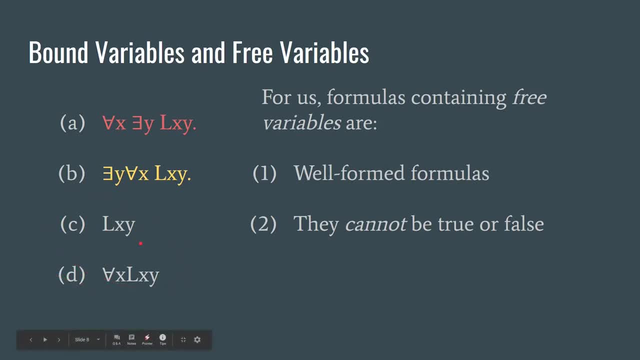 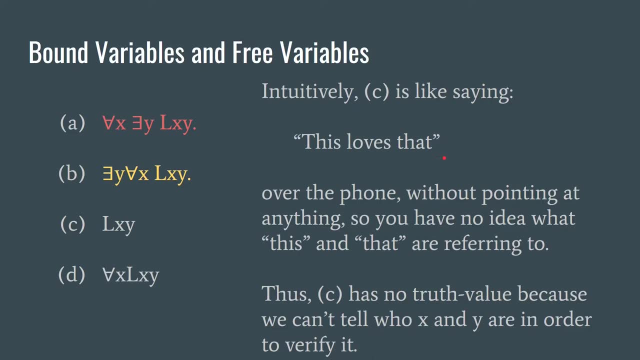 the truth or falsity of these. Let's say a little bit more about why that's so. Intuitively, C is like saying this loves that, So you have no idea what this and that are referring to. So if I just tell you this loves that, you have no way of deciding what this and that are referring to. 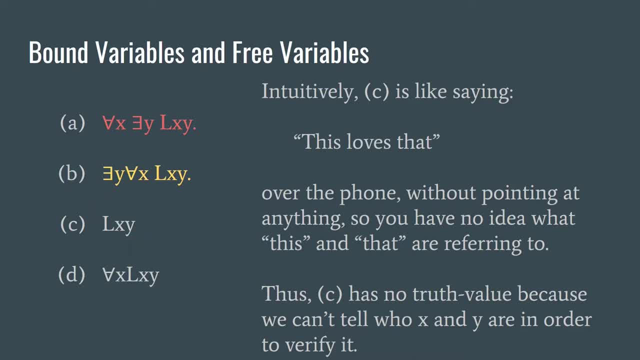 There's an indeterminacy here, So this doesn't create a sentence that can be true or false. C has no truth value because we have no idea what x and y are going to stand for. So these are called propositional functions, Because if we did substitute a name, 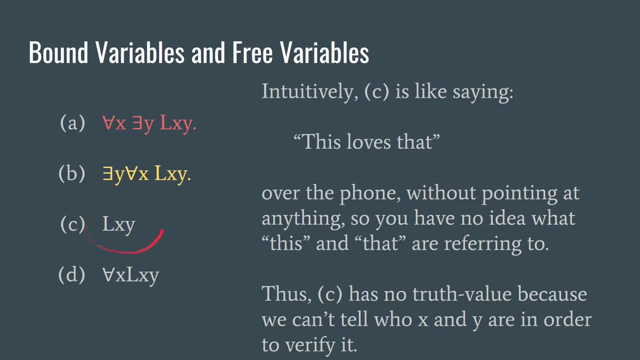 name for these, then we could determine a proposition. So suppose we put in for x and and for y bill, then we have and loves bill, then we have a proposition. So formulas with free variables are called propositional functions because they're functions from the domain of 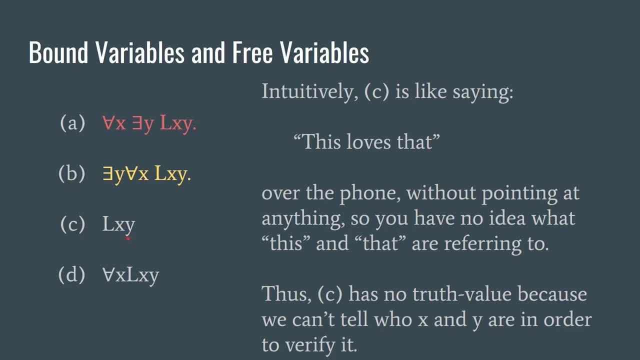 objects to a proposition. If we were to complete this indeterminate proposition by plugging in names, then we would get a proposition fully determined. So this is called a propositional function. Same thing here. any, any formula with any free variables, even if some of the variables 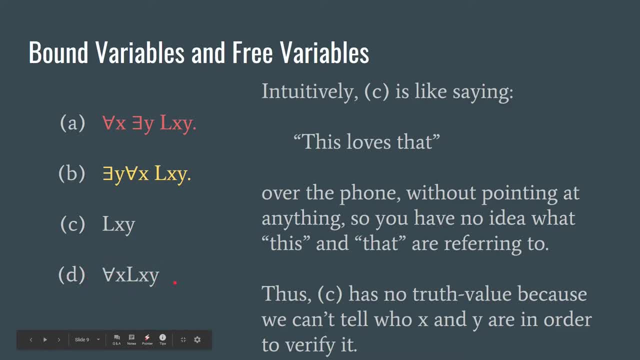 are bound is a mere propositional function. it stands in need of being turned into a fully fledged proposition. Now there are two ways to do that. One way is we could go into C and put in and for x and bill for y, or 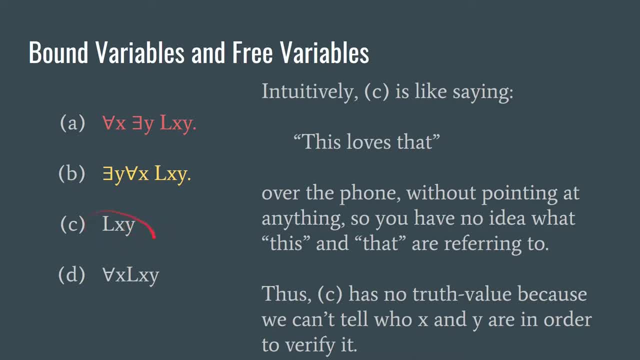 choose the whatever names you want. The other way to turn this into a fully determined proposition is to bind each of the variables with quantifiers, as in A and B. So A and B represent fully formed propositions. C and D represent propositional functions. they're indeterminate, they stand in. 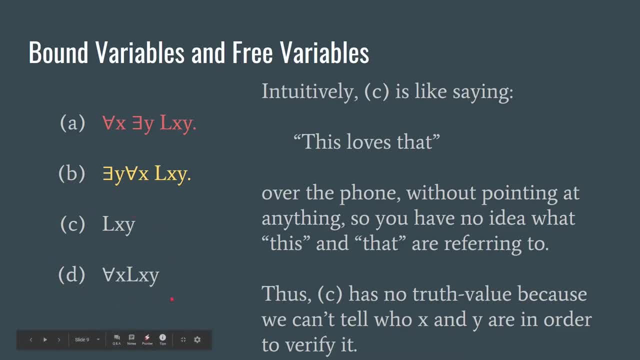 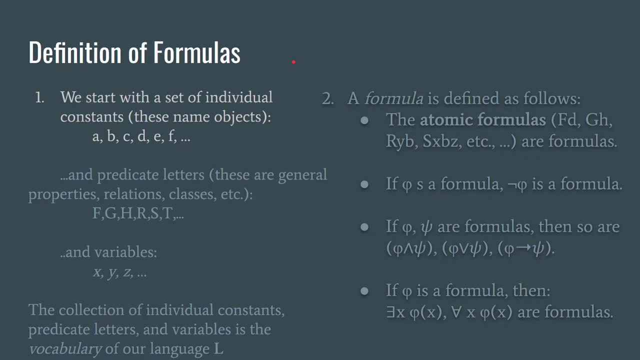 need of determination before they become propositions, But they're still well formed formulas. Now's the time to introduce our official definition of the syntax For predicate logic. this is where we define what formulas and combinations of formulas are permissible according to our formulation rules. The basic ingredients of all the formulas of 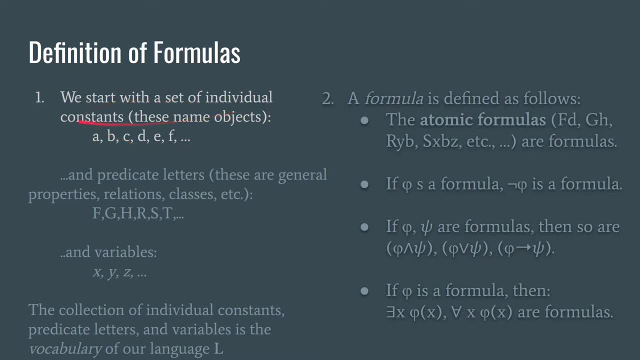 predicate logic include a set of individual constants. These constants name objects, so they're not their constant rather than variable. We then have a class of predicate letters. These are general properties rather than naming objects. they name properties, relations or classes of objects. 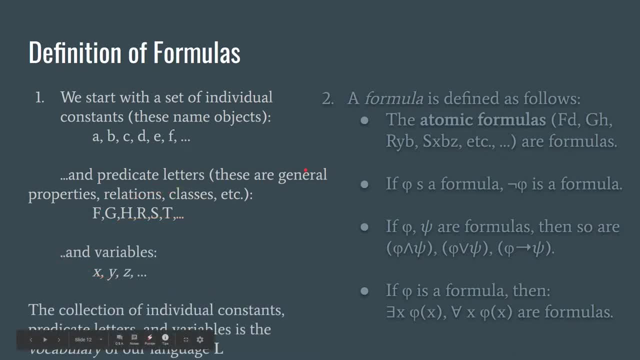 Finally, we have our variables, And this collection of individual constants, predicate letters and variables is the vocabulary, Again the ingredients out of which we can build any of the infinite number of formulas of predicate logic. Given these ingredients, we can then define formulas. 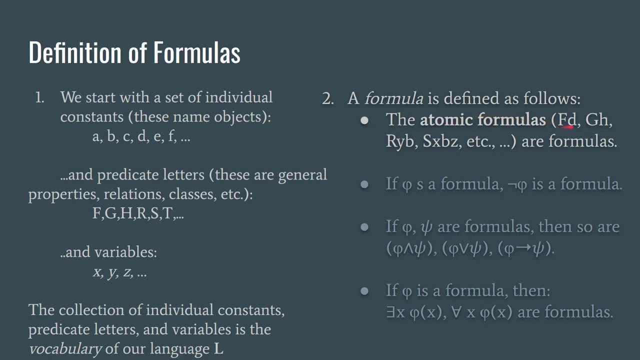 An atomic formula is something like F, D or G, H or R, Y, B. In all cases, an atomic formula is the combination of the following: of a constant or a variable with a predicate letter. Once we have this set of atomic formulas, we can then use the usual logical connectives. So if phi is a formula, then not phi is a formula. 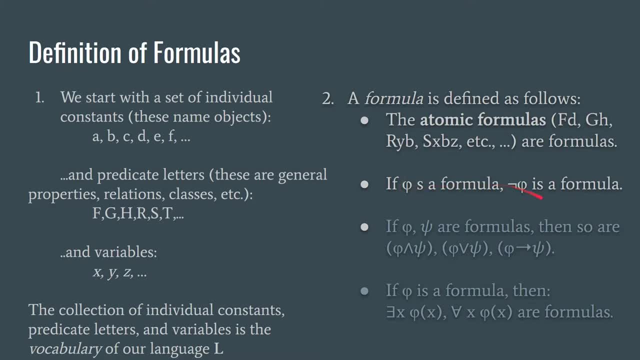 Anytime you have a well-formed formula, however complex, you can stick a negation in front of it and get a new formula. We're all familiar with the two-place logical connectives: We have conjunction, we have disjunction and we have the arrow. Anytime you have a well-formed 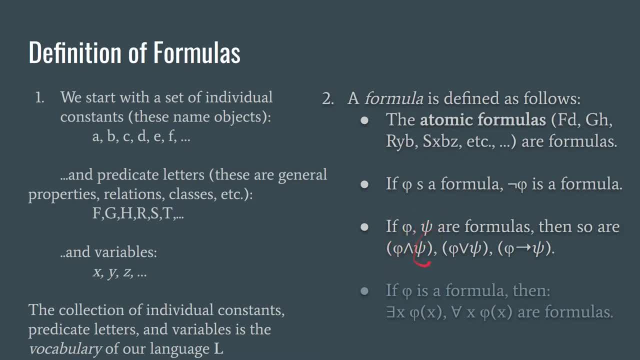 formula phi and a well-formed formula psi, no matter how internally complex these are. you can stick a conjunction in between, you can stick a disjunction in between, or you can stick an arrow in between and you get a new well-formed formula. 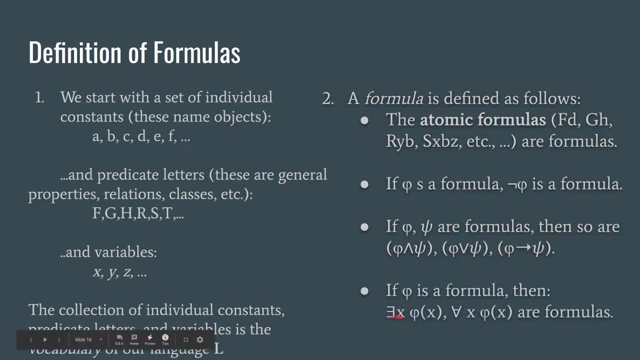 The big new thing here, then, is the quantifiers. If you have a well-formed formula with a free variable- you can stick a disjunction in between, or you can stick an arrow in between, or you can stick a variable in it- then you can bind that variable with the quantifier. 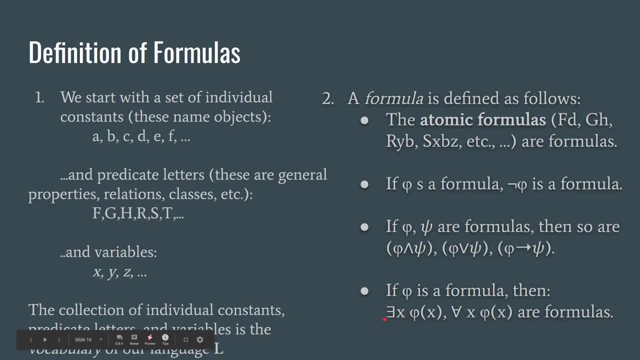 that is to say, stick a quantifier in front of it. Now notice: phi x might already contain other quantifiers. That's okay. We can do multiple quantifiers with a nested depth. That's one of the brilliant, powerful aspects of this new mathematical logic. as opposed to, 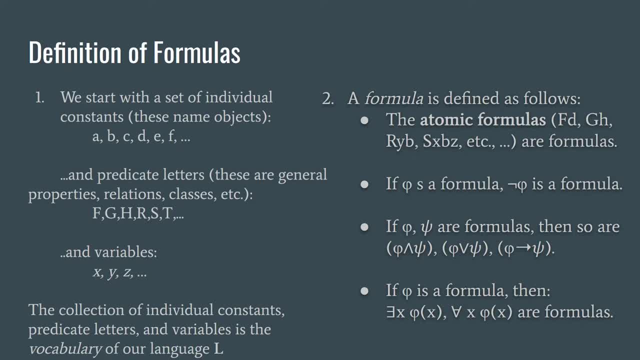 anything that came before. Now. one restriction on this is that notice phi. x is a formula with x free. If x is already bound by a quantifier, we cannot just stick another quantifier in. Suppose phi is shorthand for for all x, fx. Well, in that case x is not. 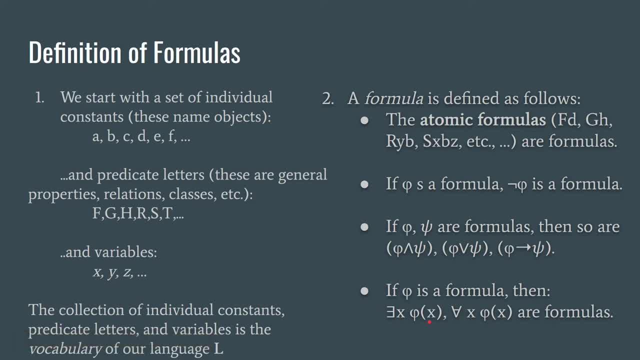 free x is already bound by the universal quantifier. so we're not allowed in that case to just stick an existential quantifier there, because then we don't know which variable is binding x. So the key here is that when you have a formula with a free variable x, then you can bind it. 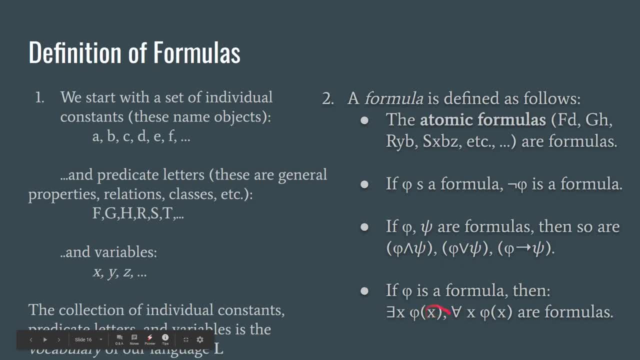 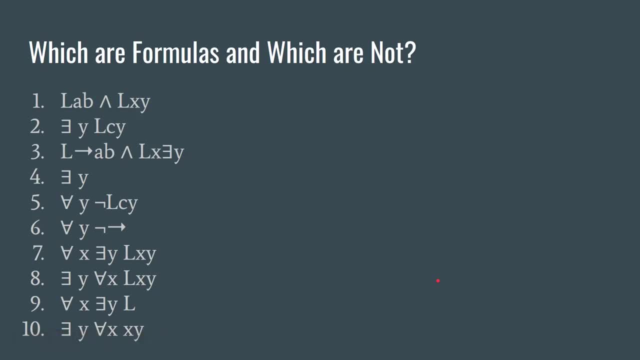 with a quantifier, But if that variable is already bound, then you can't rebind it with a new quantifier. So here's a little exercise. If you want to pause the video and carry out this exercise, that would be advisable. What you want to do here is look at these formulas. 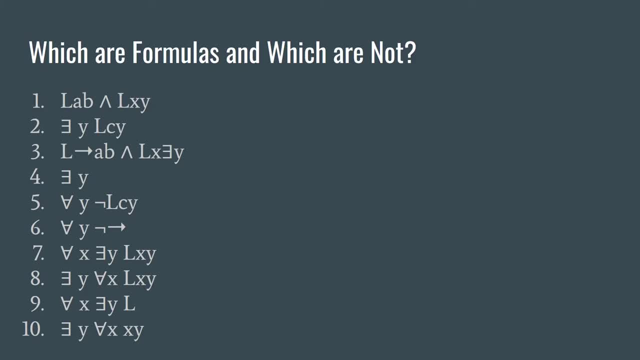 and, based on the formulation rules that we just went over, decide whether these are well-formed, which ones are well-formed, which ones are not. Well, here's the answer. All of the ones in red are not well-formed. Notice in number three. we have a couple of things wrong here. We 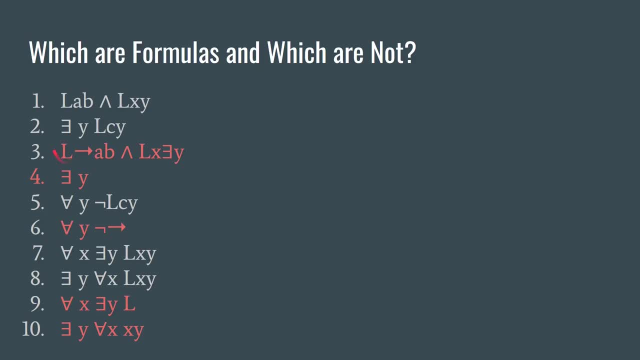 have a predicate letter with no name or variable attached to it. so you can never just have a freestanding predicate letter without a smaller lowercase name or variable. And then we have here two individual constants, a and b, with no predicate letter. So individual constants belong.